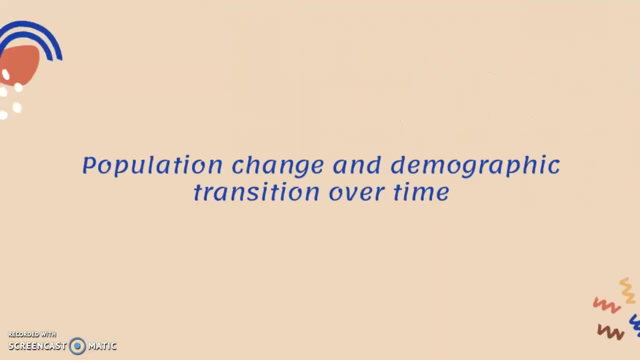 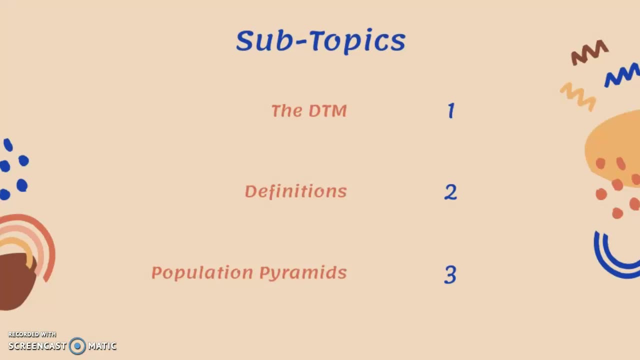 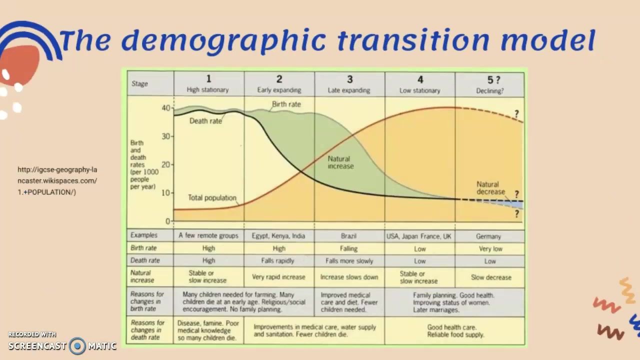 Okay so this video is about population change and demographic transition over time. So the subtopics here in this part of the syllabus are the demographic transition model, some key definitions and population pyramids. Okay so this is the demographic transition model, and the link at the side is where I've gotten this diagram from. So there are five stages of 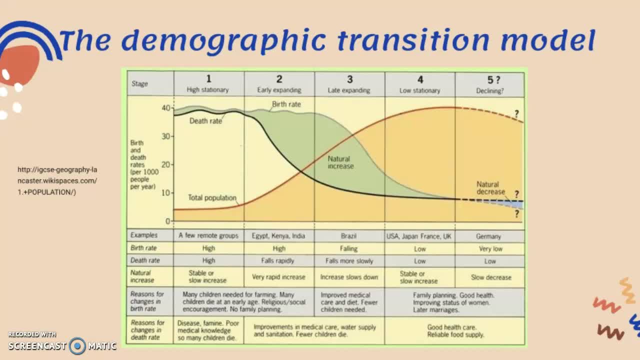 the demographic transition model and these are kind of the key points about each of the stages. So in stage one the birth rate and death rate is very high and there's kind of a slow and stable natural increase. Natural increase is, of course, the difference between 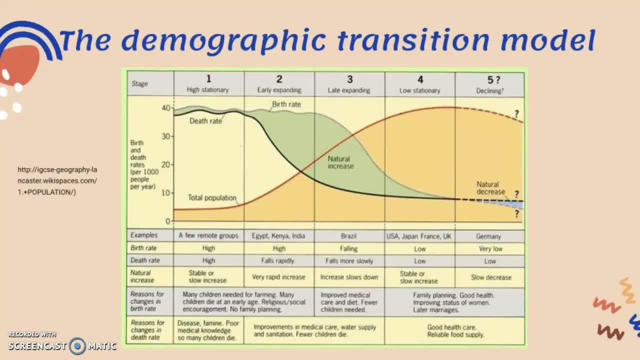 the death rate and the birth rate, which either makes the population go up or down. however, you must take into account that migration does impact population and is not accounted for in this model, so that's kind of like a weakness of the model. Okay, so there's a lot of disease, high birth rate people are not aware of kind of. 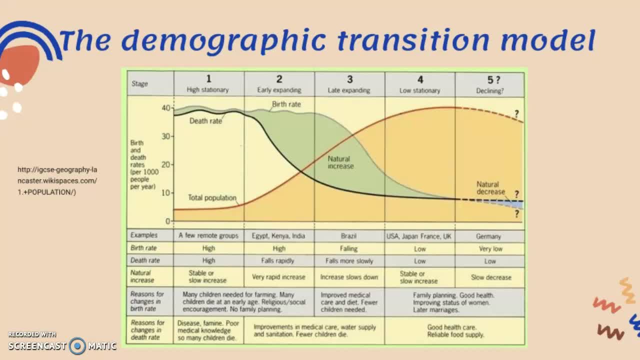 the idea of health and disease. so, yeah, okay, and then we come to stage two, and because healthcare kind of begins to improve and sanitation arises, the death rates begin to fall, but birth rates still remain high. so, um, the population does start to increase at a much. 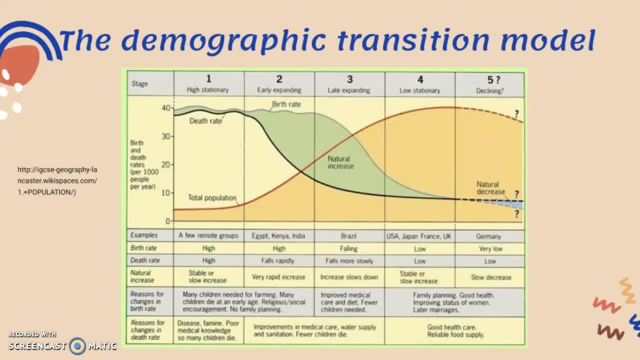 more rapid rate because death rates are low. birth rates are high, of course, okay. and then you move on to stage three, when birth rates do also begin to fall because of improved knowledge about kind of health and medical care and their kind of cultural norms change, where less children are needed. 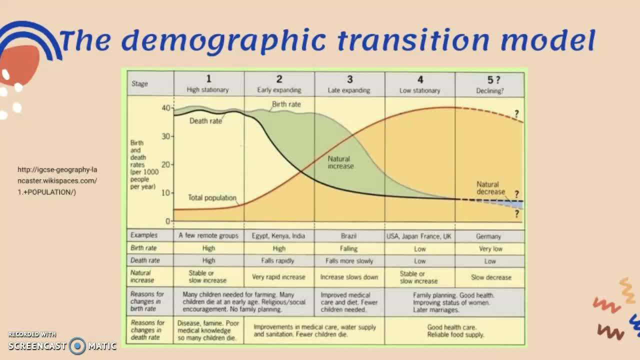 because they're not seen as kind of an economic asset as they would be in many kind of developing or less developed countries. so here we see that the increase, um, the natural increase as shown by the orange line, kind of becomes less steep. okay, and then we move on to stage four, where both the 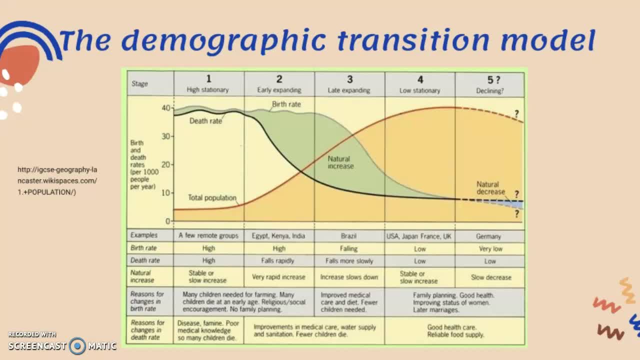 birth rate and the death rate are low. but the birth rate is still higher than the death rate. that's very important because the population is still increasing just very slowly, as you can see by the orange line. and then we move on to stage four, where both the birth rate and the death rate 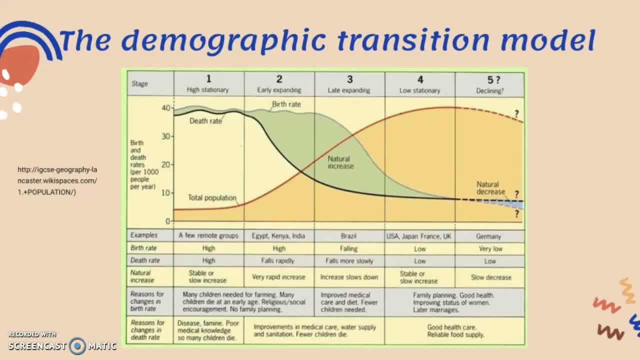 in stage four it's kind of it's coming kind of to a plateau, but not fully, um, and this is because of family planning, improved status of woman, later marriage, etc. okay, and then we get to stage five, which is basically said to be a stage in which the birth rates fall below the death rates. so 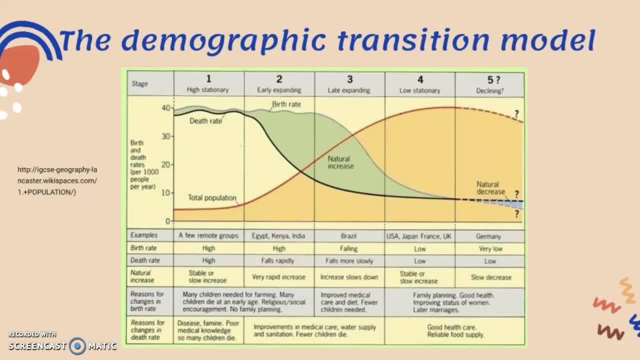 there's a natural decrease instead of a natural increase, because there's more people dying than then being born, um which, you know, than the population would fall again. this is very typical in many high-income countries such as japan, which is a good example of a very large asian population. okay, so this is the 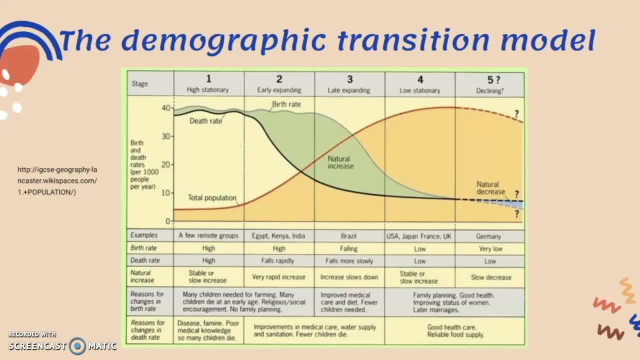 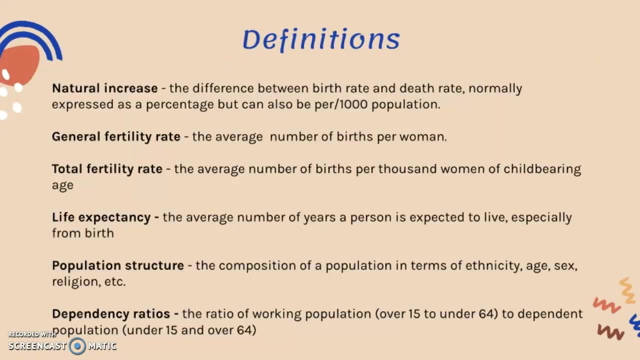 transition model that you should know each stage and kind of why each different stages look the way they are, but also remember the criticisms, such as it doesn't account for any migration, immigration and immigration aren't included. okay, so here are some very important definitions: natural increase, as i mentioned, the difference between birth rate and 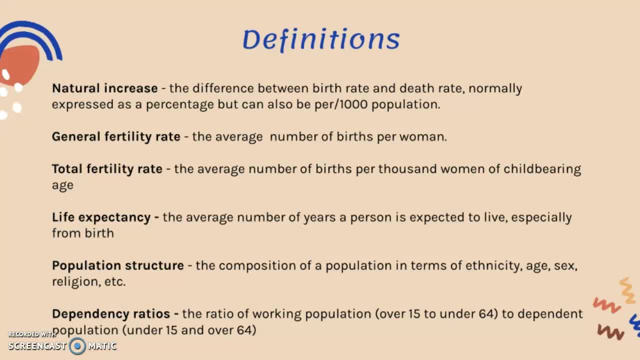 death rate, normally expressed as a percentage, but can also be per thousand of the population. um, and if it's a natural decrease, of course that means the death rate would be higher than the birth rate. but if it's increased, the birth rate is higher than the death rate. okay, general fertility. 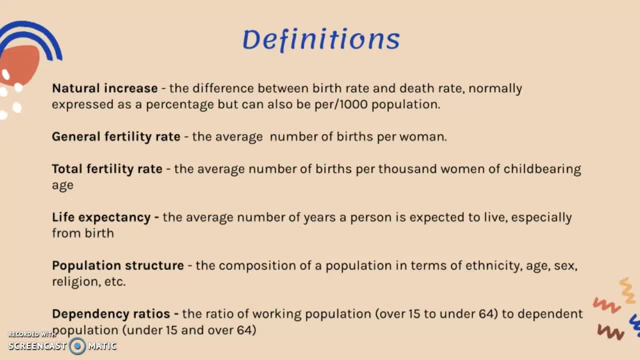 rate is the average number of births per woman. total fertility rate is the average number of births per thousand women of childbearing age. so make sure you know the difference between those two. um, you know it's per woman or per thousand women. okay, and then life expectancy is the average. 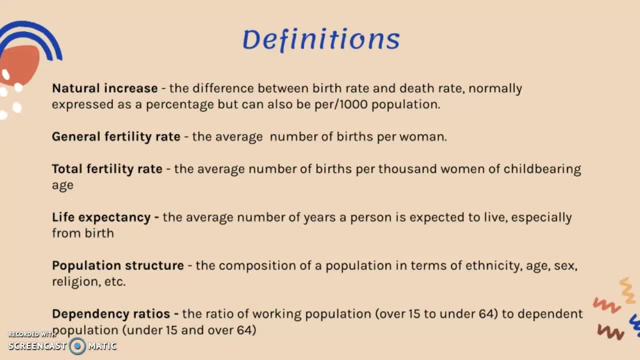 number of years a person is expected to live, especially from birth. population structure is the composition of a population in terms of ethnicity, age, sex, religion, etc. finally, dependency ratios is the ratio of the working population. so the working population are those over 15 and under 64, so that whole bracket to dependent populations, which are the young.